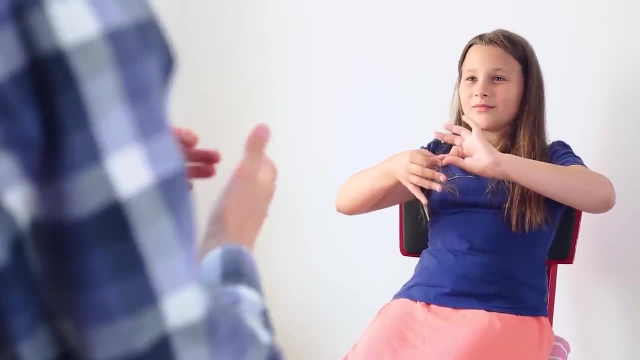 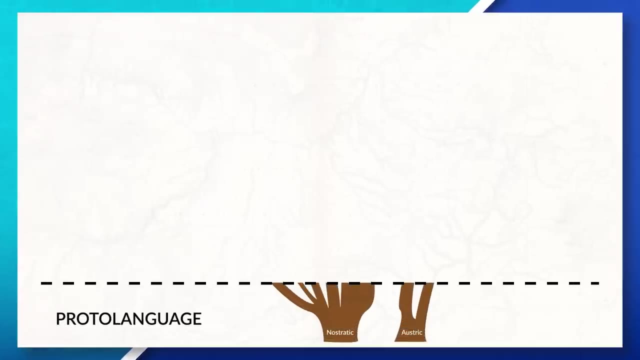 languages. we can go back in time and trace a language back to its origin. When we go back to the starting point of a language, we are looking at a proto-language. Oftentimes this means we are looking back in time before written records. From there we can move up. 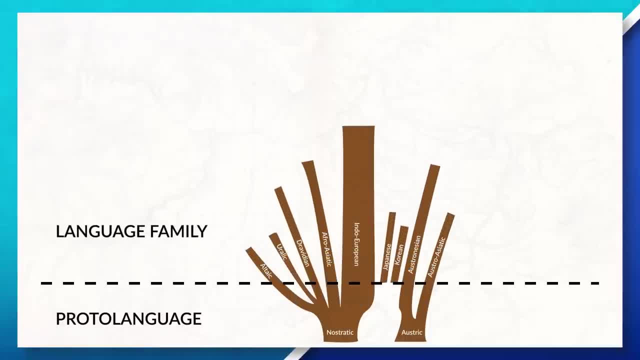 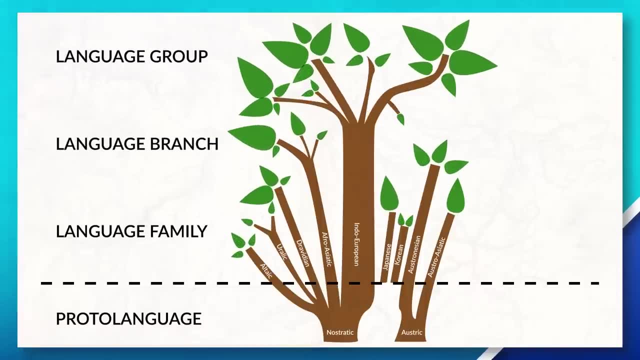 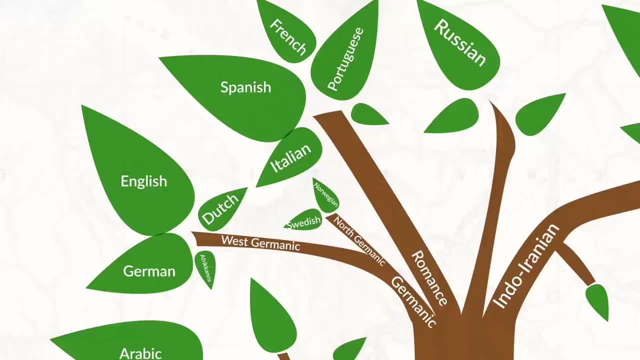 to a language family, which consists of a variety of different languages that have a common ancestry. Think of it as if the languages are genetically related. Then there are the language branches or groups. A language branch is a cluster of different languages that are part of a language family and make up a subdivision of that language family. A language group: 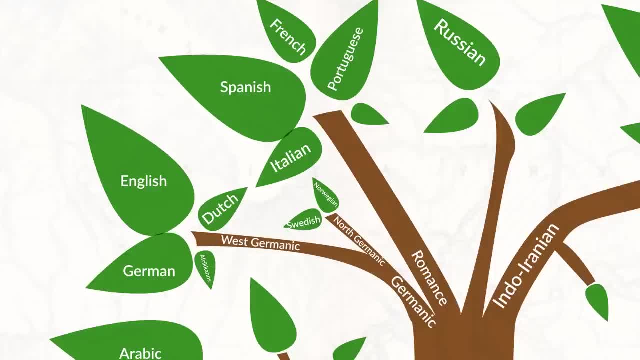 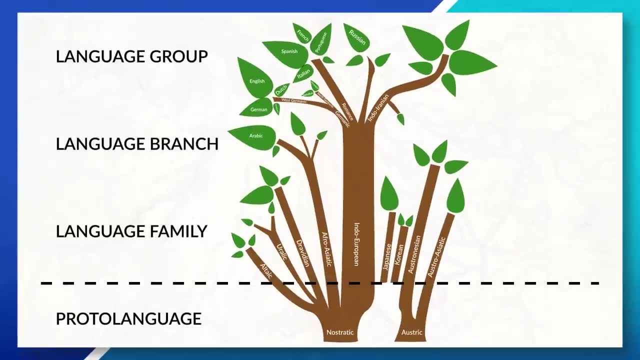 on the other hand, is made up of different languages that are part of a language branch. These languages often have similar vocabulary and grammar. For example, we can look at Indo- European as an example of a language family. Here we can also see examples of language. 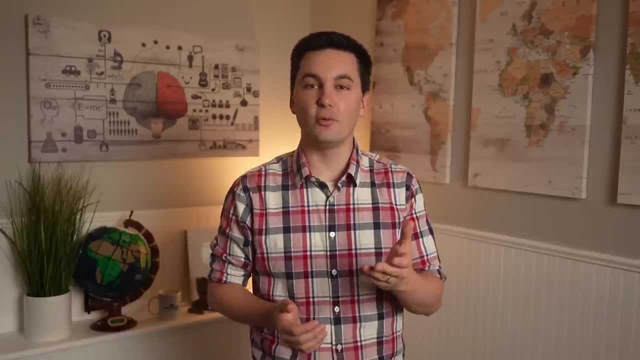 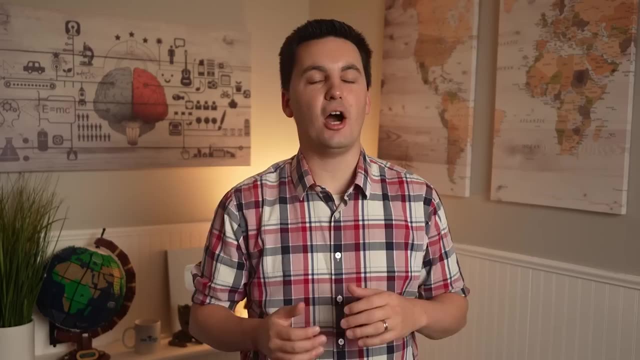 branches and also language groups. One of the interesting aspects of languages is how they evolve over time. As different people and cultures interact, we see languages shift and evolve. Oftentimes, words may take on new meanings. For example, English is one of the. 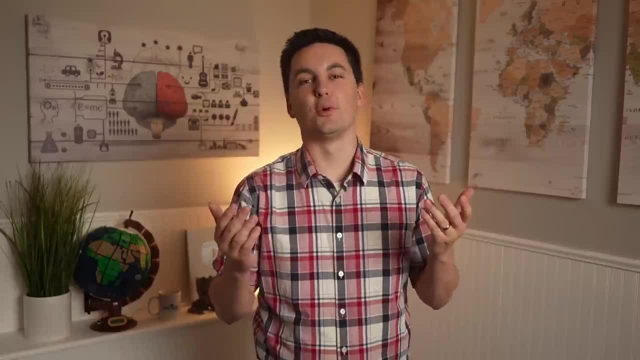 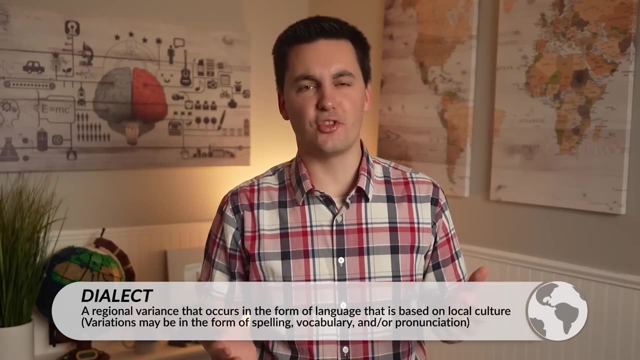 most commonly spoken languages in the world today. Depending on where you are located, you will often hear different dialects spoken and hear different words take on different meanings. A dialect is a regional variance that occurs in the language family. A dialect is a regional variance that occurs in the language family. 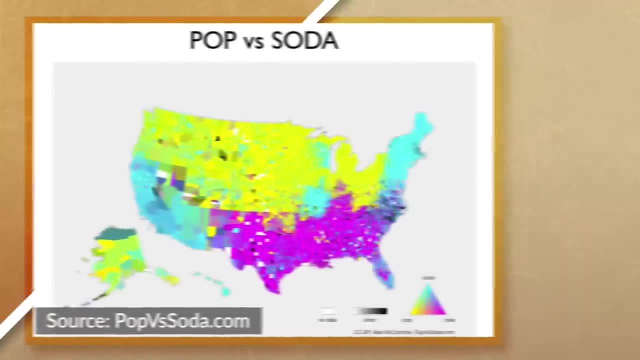 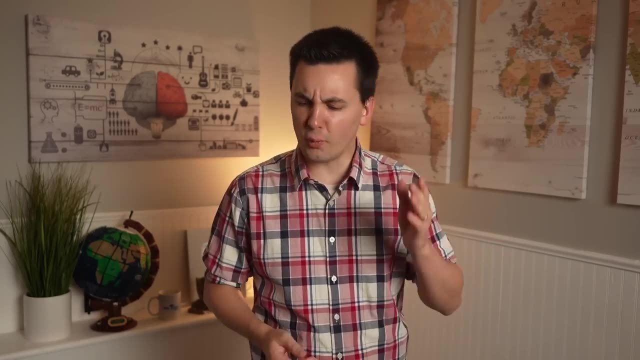 A dialect is a regional variance that occurs in the language family. It is often based on the local culture. Dialects can be differences in the spelling, vocabulary and or pronunciation of certain words. For example, I am from Minnesota and here we drink pop, not soda, And when. 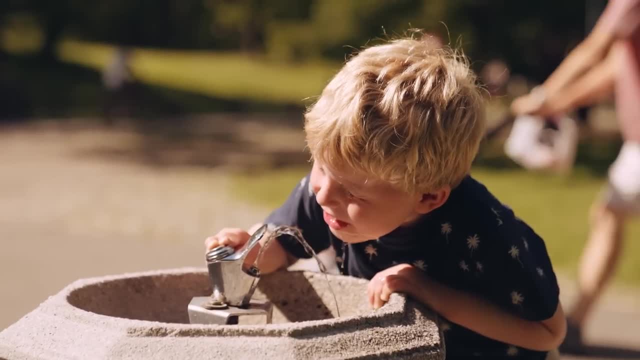 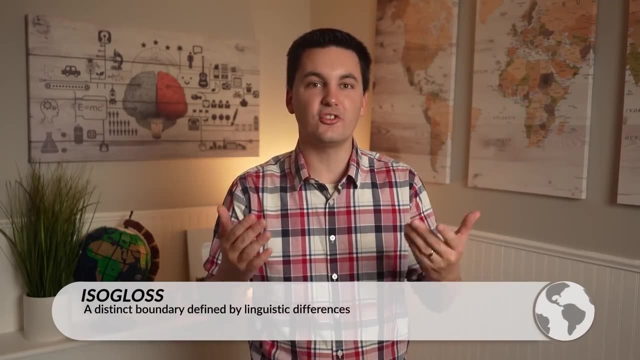 we need to get water, we go to the drinking fountain, not the bubbler, And we sometimes eat hot dish, which is essentially a casserole. Now, sometimes regional differences are so distinct that we could see the formation of an isogloss, which is a boundary that is based. 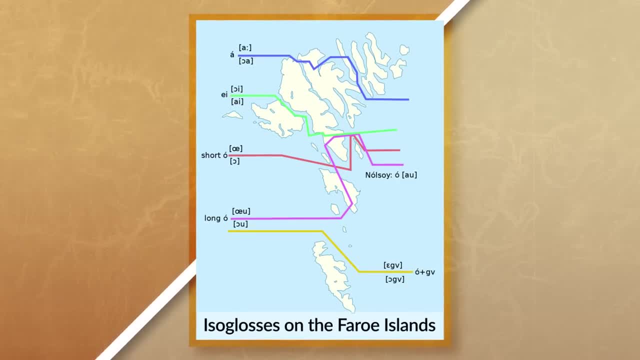 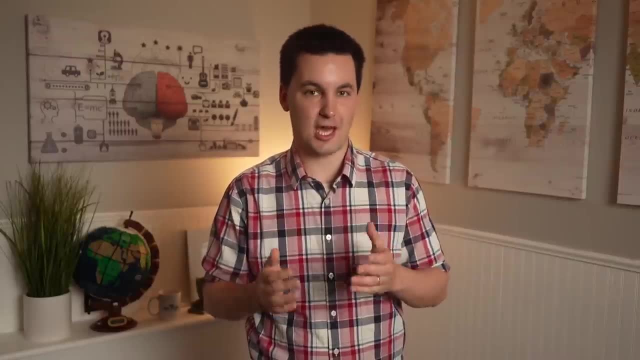 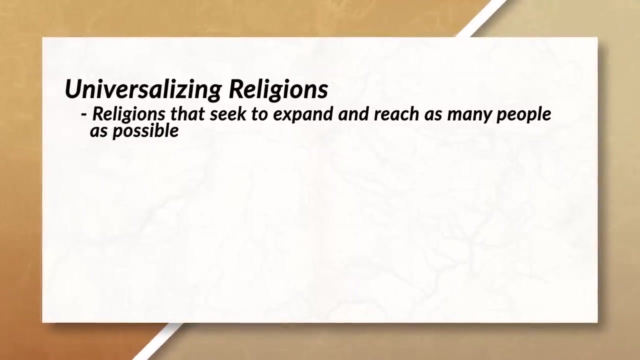 on linguistic differences. Speaking of differences between different regions and locations, we can also look at how religions differ from location to location. When looking at religion, we can see two main categories: universalizing religions and ethnic religions. Universalizing religions are religions that seek to expand and reach as many people. 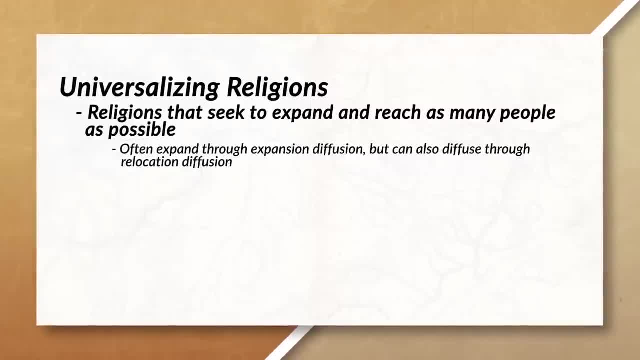 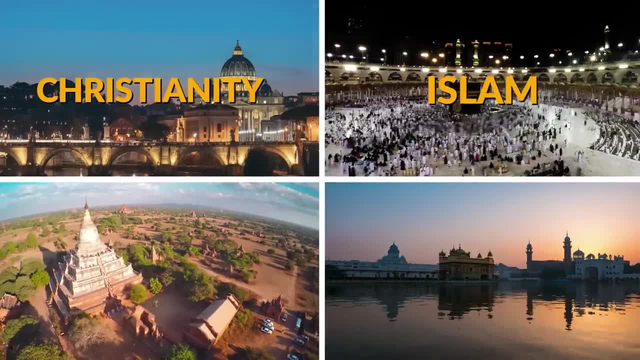 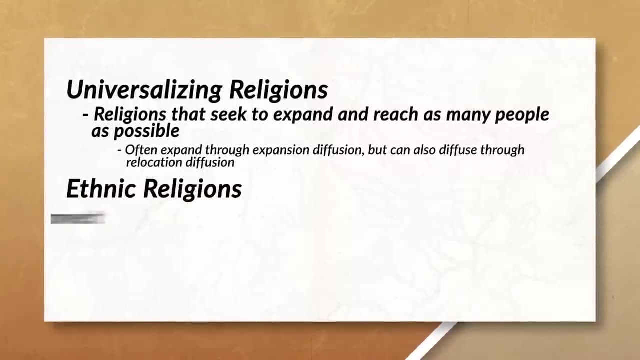 as possible. Oftentimes these religions will expand through expansion diffusion, but can also diffuse through relocation diffusion. In this video we will be just scratching the surface on Christianity, Islam, Buddhism and Sikhism. All are examples of universal religions. We also will examine ethnic religions as well, which often stay in one location. 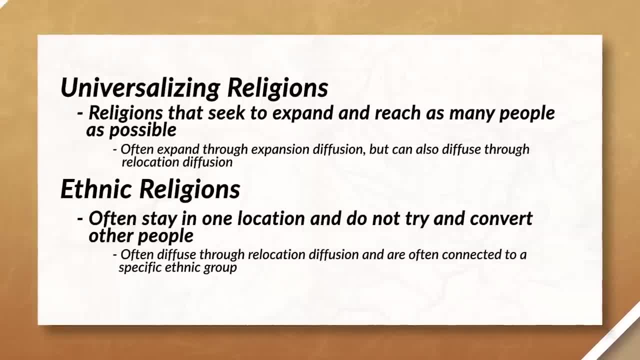 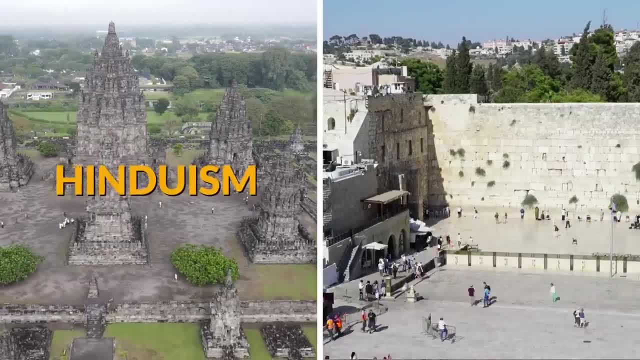 and do not try to convert other people. These religions often diffuse through relocation, diffusion, and are often connected to a specific ethnic group. The two ethnic religions we will talk about in this video are Hinduism and Judaism. To start, let's go back to universalizing. 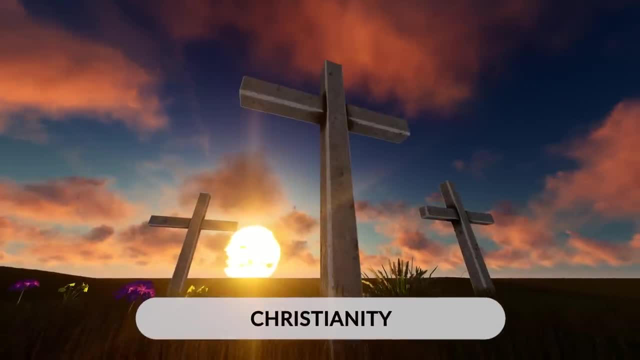 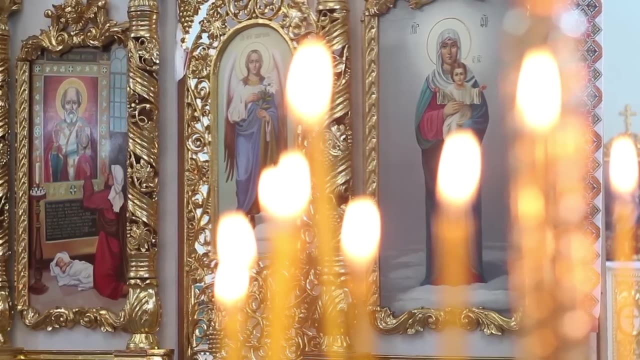 religions and look at Christianity. Christianity's hearth is located in the eastern Mediterranean. It's a monotheistic religion, meaning they believe in one God. This is one of the Abrahamic religions and stems back to the teachings of Jesus Christ. Christians believe that Jesus. 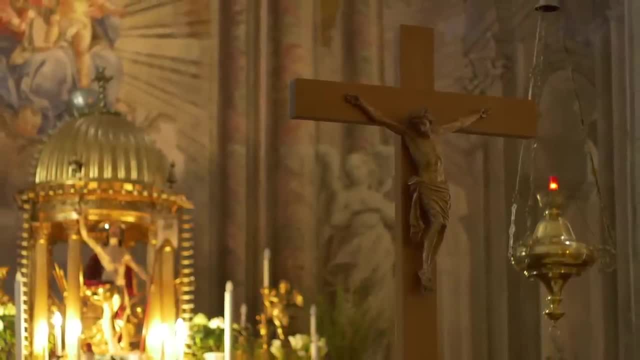 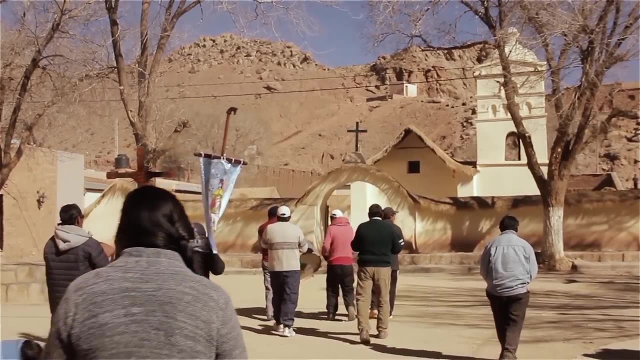 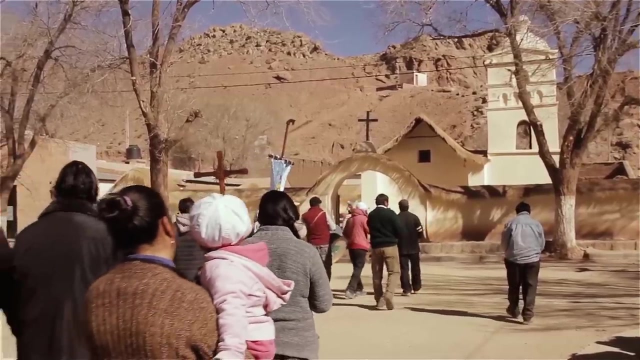 was the Son of God, who was sent to earth to save humanity and die for our sins. Their important religious texts are the Bible and the Ten Commandments. Christianity diffused around the world through a variety of different ways. We could see hierarchical diffusion due to missionaries and boarding schools that worked to convert people to the faith. Colonialism- 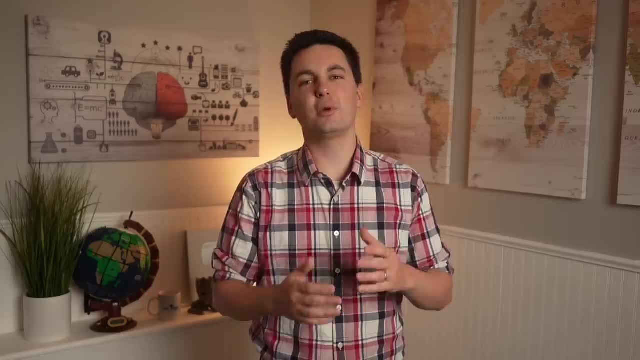 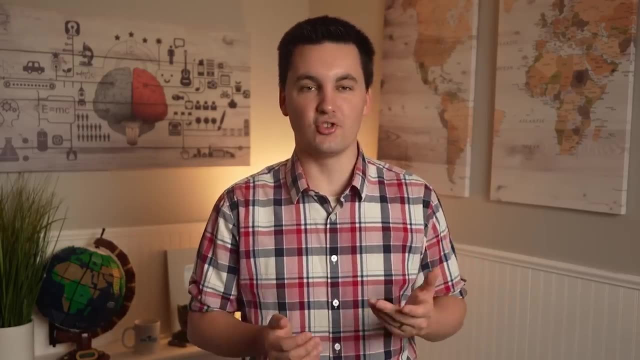 and imperialism also helped spread the faith to new lands And relocation. diffusion occurred through migration of people. The religious texts are the most important religious texts in the world. Another Abrahamic religion that is also a universalizing religion is Islam, which has its hearth located in the eastern Mediterranean. Islam is a monotheistic 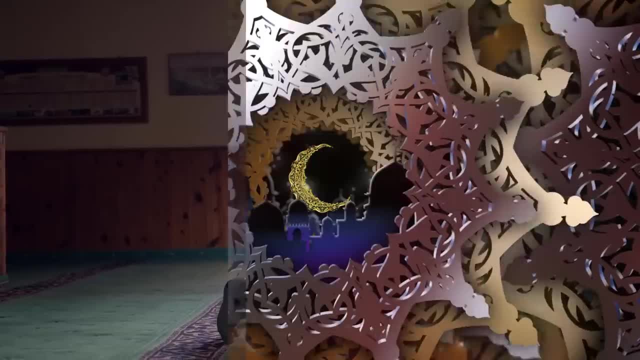 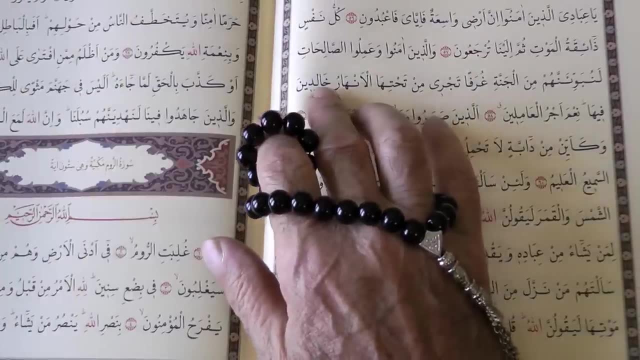 religion and is traced back to its single founder, Muhammad. After Muhammad passed, the faith became split between the Shia and Sunni. The split was over. who should lead the faith? Both the Shia and Sunni used the Quran as their holy book and followed the 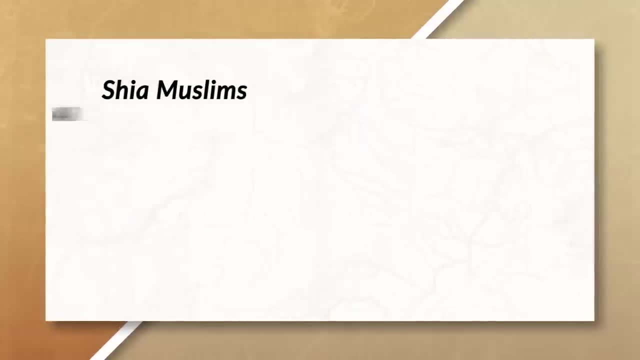 five pillars of Islam to help guide their daily lives. The Shia accept the descendants of Muhammad's son-in-law, Ali, as the true rulers of Islam. Islam is a religion that is based on the religion of Islam. The Sunnis, on the other hand, wanted Muhammad's successor. 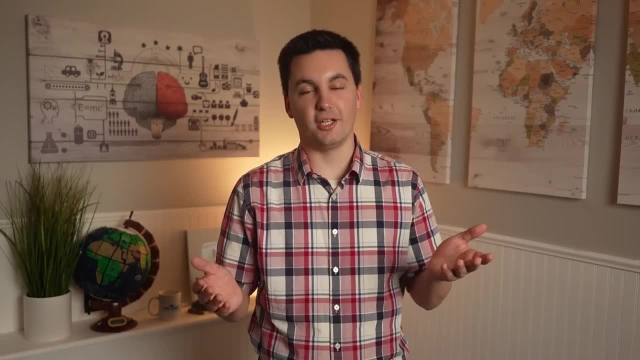 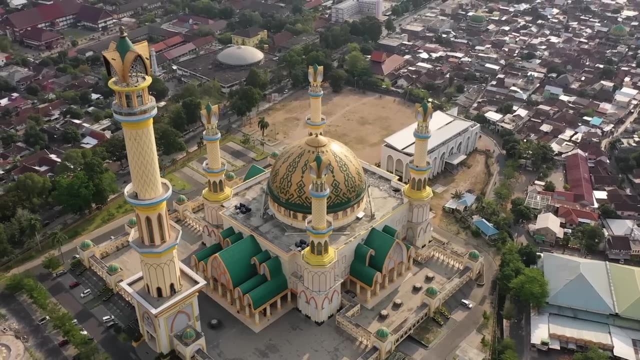 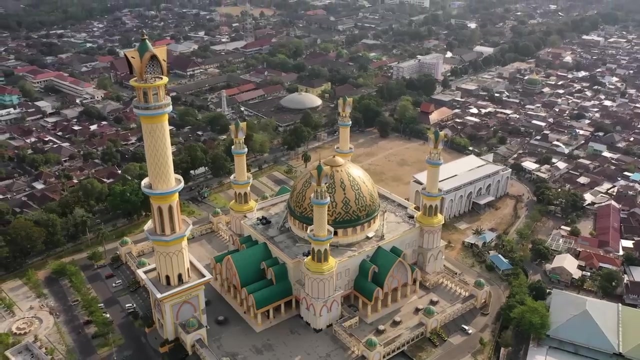 to be chosen by a community of his followers. Similar to Christianity, Islam has diffused in a variety of different ways. We could see examples of hierarchical diffusion as Arab traders and missionaries moved through the Middle East and to Africa, bringing new goods and wealth to different bazaars. As the traders and merchants moved through the area, they 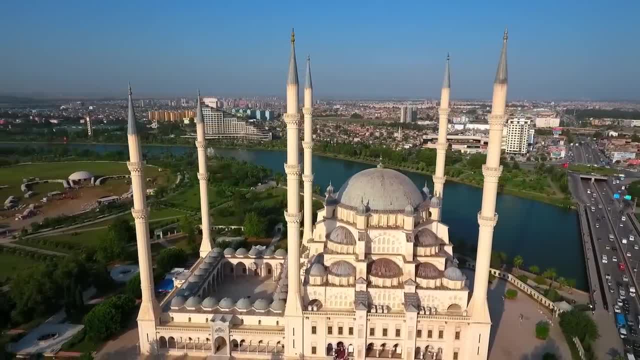 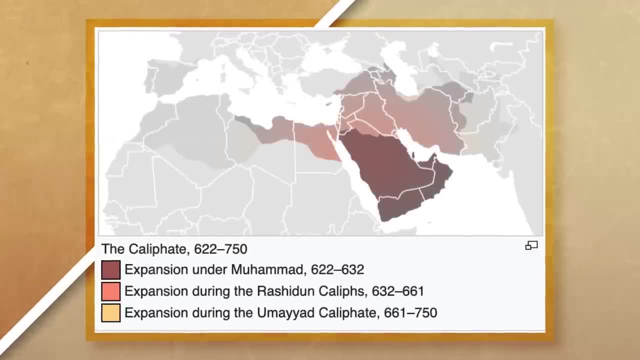 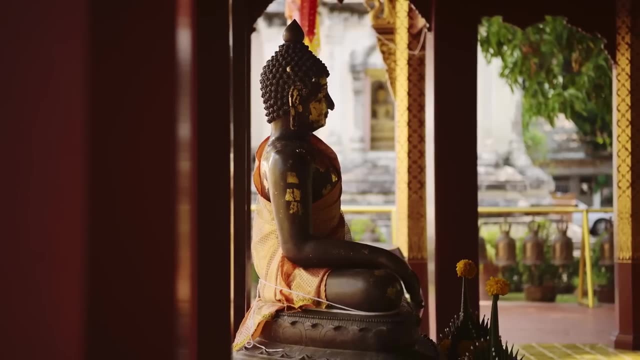 would explain to people that it was Islam that allowed them to become so prosperous. We could also see diffusion occur through relocation, diffusion due to the migration of people, And also diffusion occurred due to trade and war as the Islamic empire grew and expanded over the course of history. Moving into South Asia, we have Buddhism. 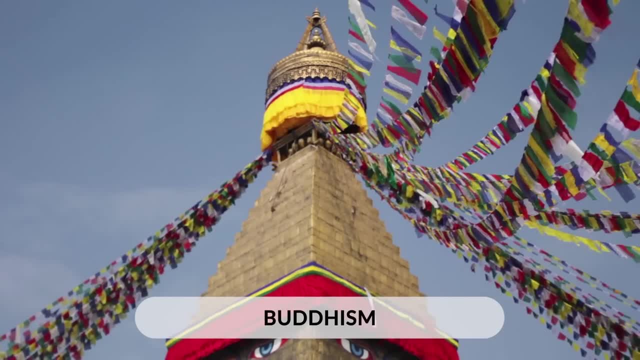 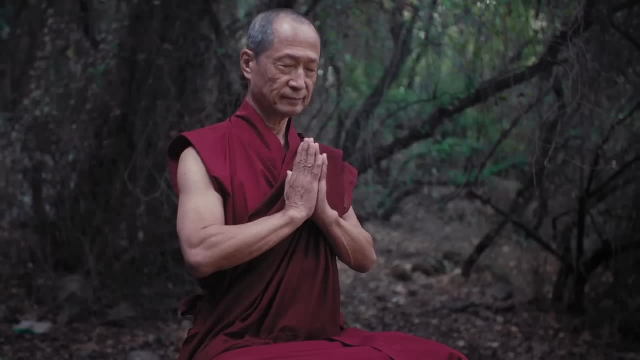 which, unlike the previous two religions, does not have a set deity. Buddhism was created by Siddhatra, also known as the Buddha. Buddhism believes that anyone can reach salvation by following the Four Noble Truths and the Middle Path. People can break free of their material. 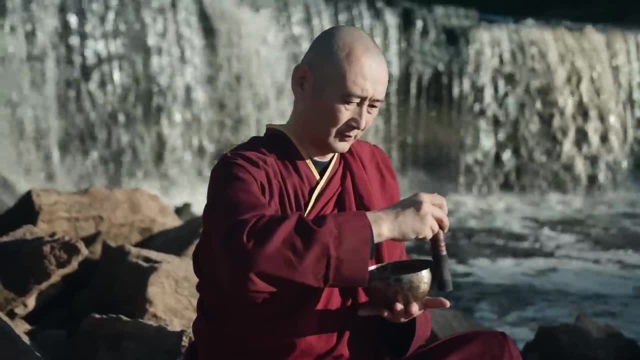 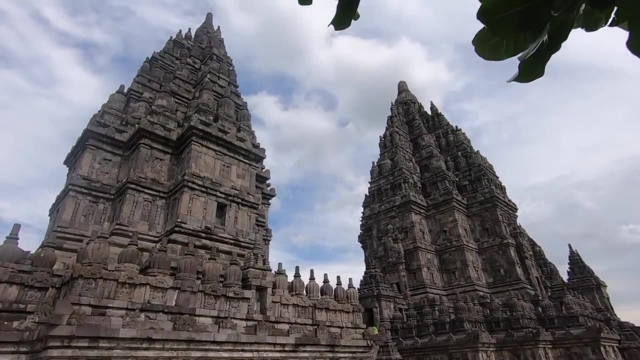 needs and become free. This faith gained in popularity due to the belief that everyone could reach salvation In Buddhism. the predominant religion of the region was Hinduism, which had connections with the caste system and did not preach salvation for everyone. This allowed for contagious 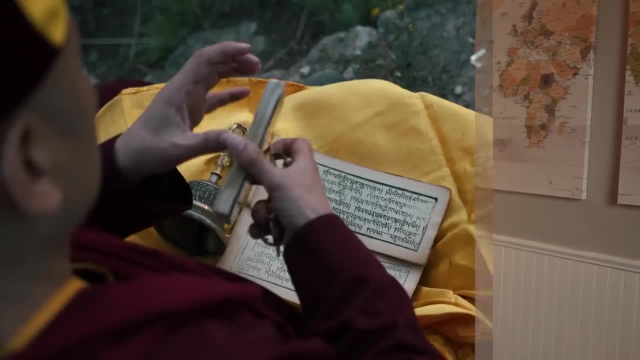 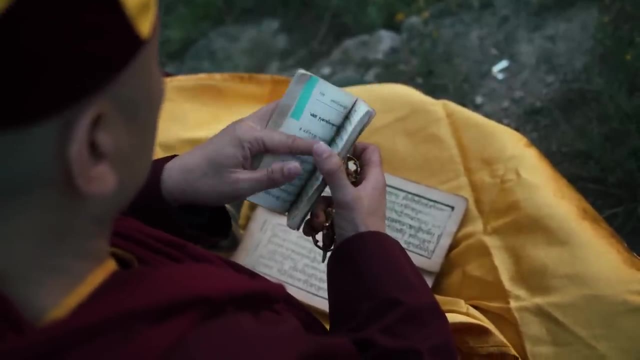 diffusion to happen as Buddhism spread throughout communities. We also saw relocation diffusion occur due to the migration to other countries and also missionaries relocating to other regions around the world. The last universalizing religion we're going to talk about in this video is Sikhism. The 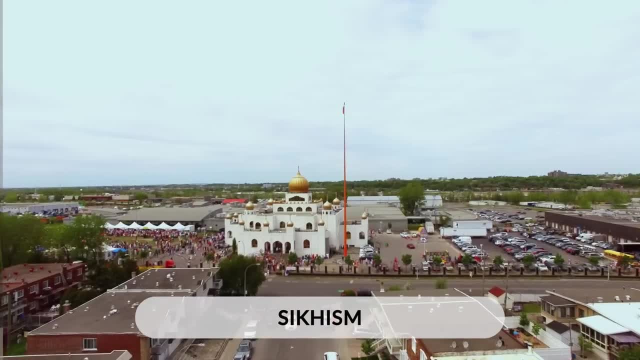 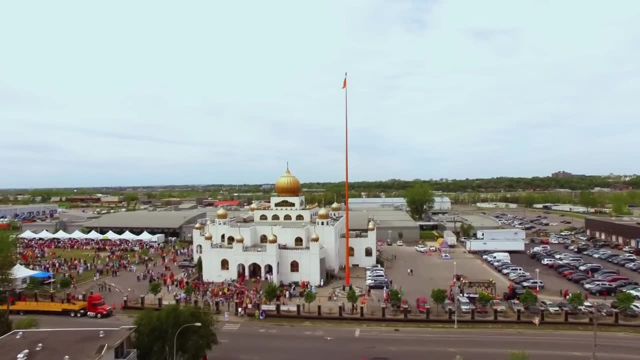 Sikhs are monotheistic and originate from the Punjab region. They diffuse through relocation andbitrity. however, their diffusion was limited due to being located between Hinduism, Islam and Buddhism In the United States and many countries around the world. people 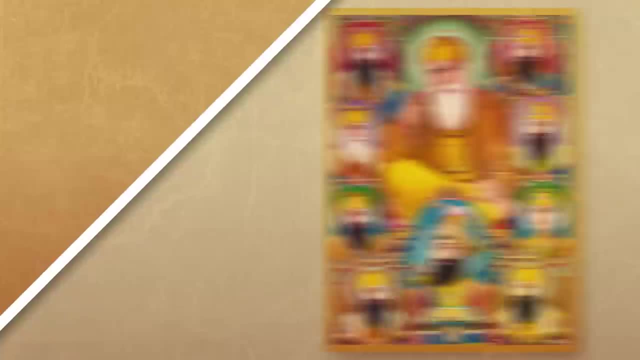 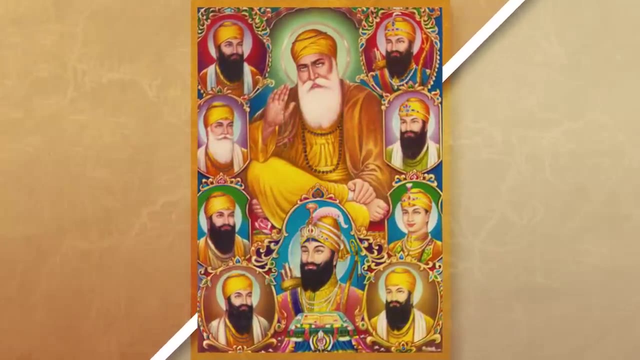 often confuse Sikhs as Muslim. However, they are very different. Sikhs believe in ten gurus who help guide Sikhs in their daily lives. These gurus preached the Word of God and helped create their holy book. Moving from universalizing religions to ethnic religions, we can see 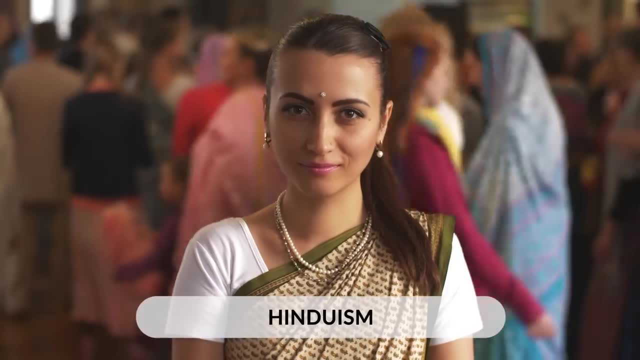 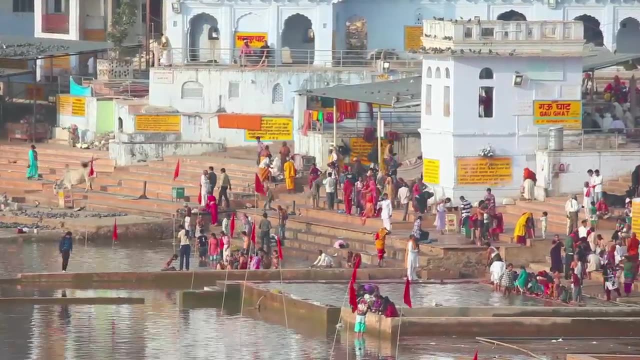 Hinduism, which originated in South Asia. Hinduism is one of the world's oldest religions. Hinduism believes in karma and dharma. The Vedas are its sacred texts and, interestingly enough, we don't know exactly who the founder of the faith is, As Hinduism spread throughout the region. 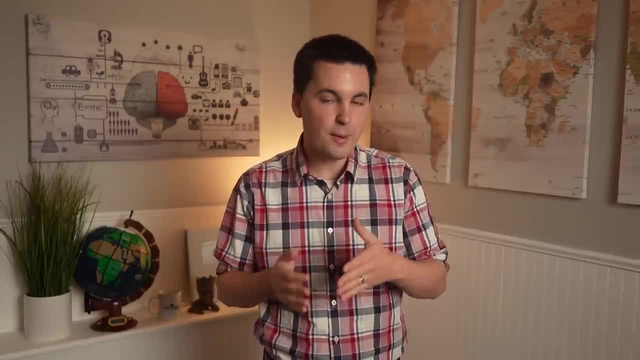 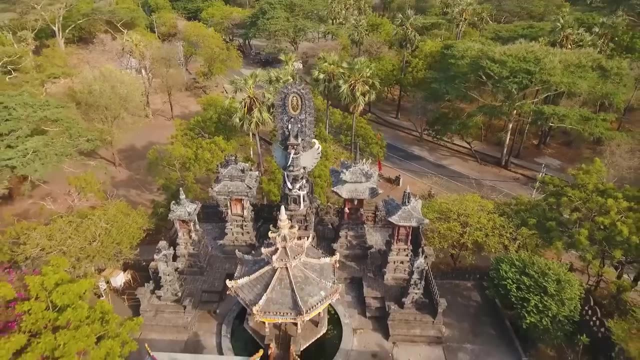 we can see it diffuse through stimulus diffusion. It would spread between different faiths, taking on some aspects of traditional faiths and eventually replacing them. We can also see diffusion occur due to the migration of people. This would be a form of relocation diffusion. 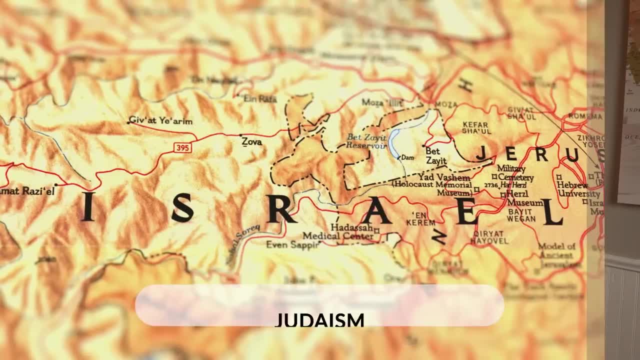 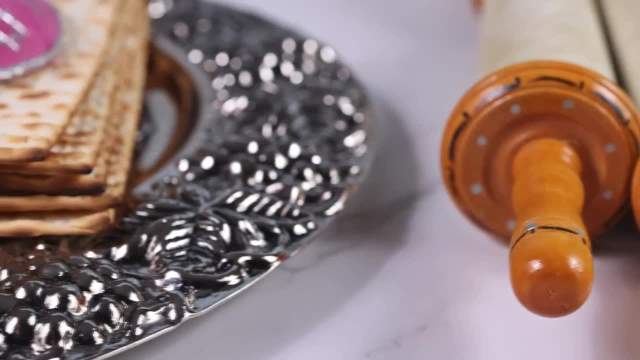 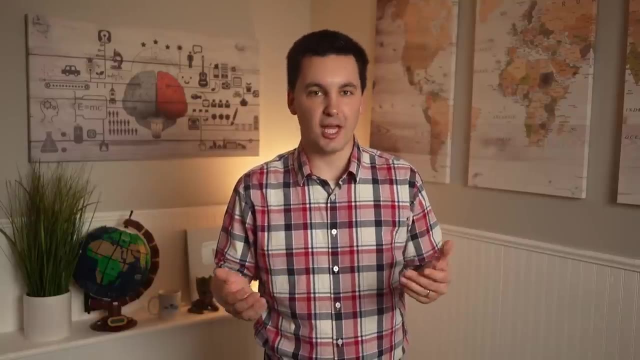 Now the other ethnic religion we are going to look at in this video is Judaism, which originated in the Eastern Mediterranean. This religion has three main branches: Reform, Orthodox and Conservative Traditions here come from the teachings of Abraham. This is actually the third Abrahamic religion. Throughout history we have seen Judaism diffused by relocation diffusion.